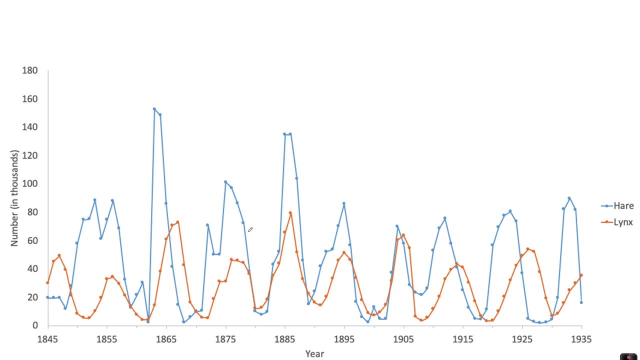 So looking into more detail at that, let's look at, for example, this section on the graph just here. You'll notice that few predators mean the prey numbers rise. So when the lynx, the orange line here, is very low, these prey numbers start to rise really rapidly. 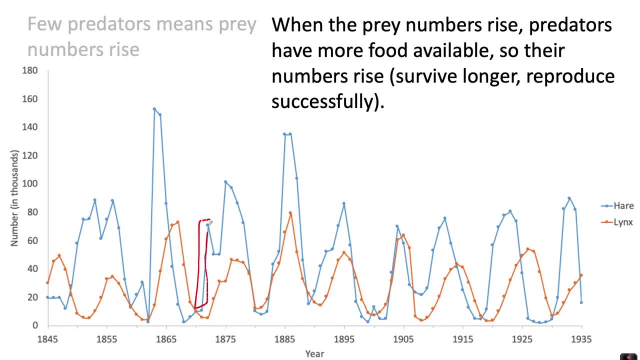 When the prey numbers rise in this section here, Shortly afterwards, the number of predators also rises. Because the prey numbers rise, the predators have more food available, So their numbers rise, And this is really calledasınax sp, And this is my fundamental objective- is to spirituality. He turns me into two individuals. And now he has seen the numbers and the prey numbers start to rise. ginguije at the old age. So when we're talking about predators, blush number would feel like, certainly not as how he before the館. be, and on the same time, I realised that prey numbers are walled up per week. kai不會 hate man понデ attempting inventing this om影ation-, but it could be to make sure the predators could have more food available. 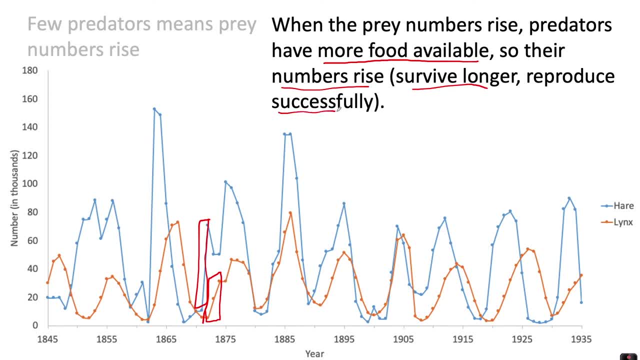 because they are surviving longer and able to reproduce successfully because of all that food that is now available. However, an increase in predators means that more prey is being eaten, and then you'll notice at this point here, these prey numbers will start to fall, because those predator numbers had got quite 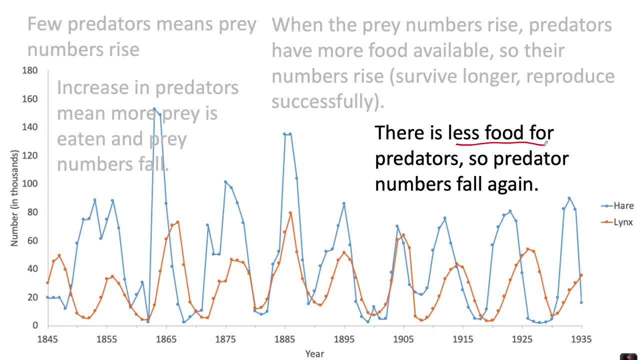 high. There is now less food for the predators, so the predator numbers start to fall again. so the prey starts to rapidly decline and then, you'll notice here, so does the lynx and that starts to fall again. and this cycle of prey increasing and predators increasing and then falling, is called a predator prey. 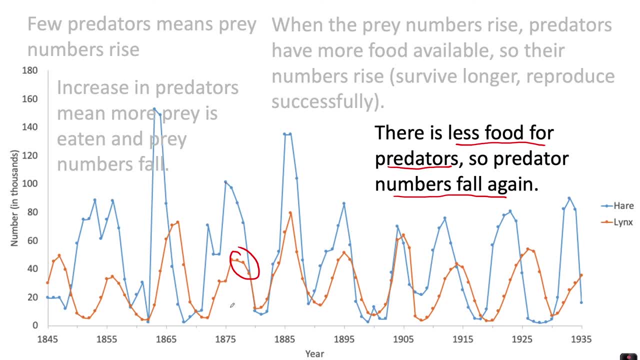 relationship and you can see that that is repeated in the predator number cycle every few years in these cycles. so the numbers of hair that you'll find is totally dependent on the numbers of links in the population and vice versa. so the number of links you'll. 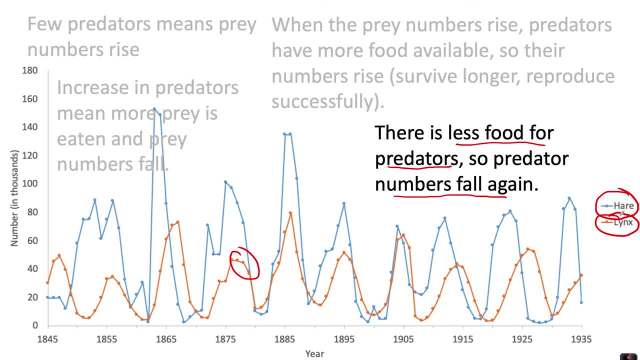 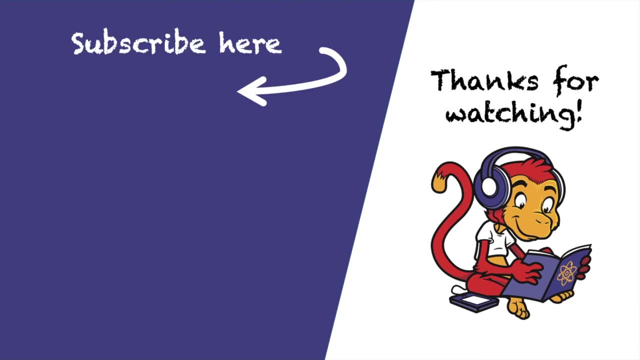 find will also be dependent on the prey that is available. hi guys, if you enjoyed that last video, then please click on the screen to subscribe. you can also find all my videos in one place at gcscrevisionmonkeycom. if you're a teacher, check out the key.